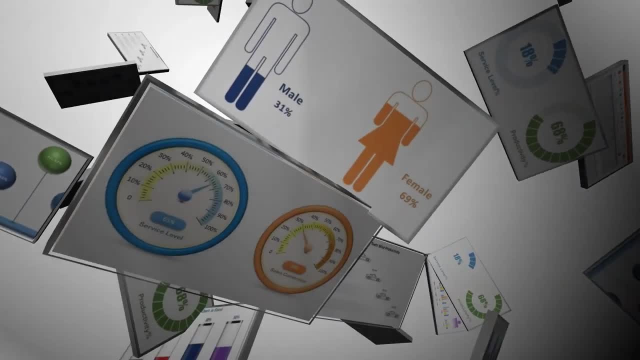 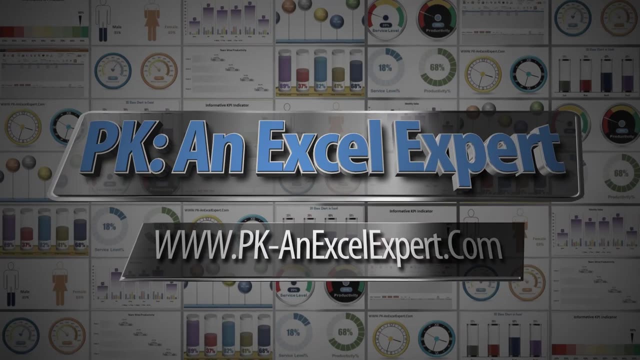 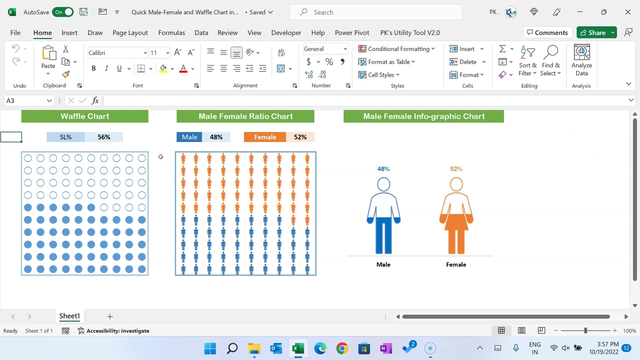 Hello friends, welcome back. My name is PK. In this video you will learn how to create the quick male-female infographic chart and a VFL chart, as well as a male-female ratio chart, And I will tell you the quick trick to create this chart in Microsoft Excel. So 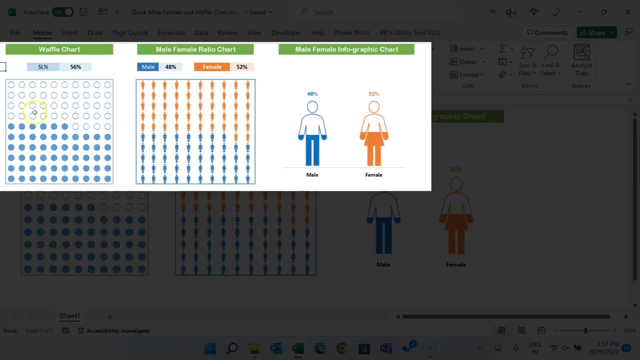 as you are seeing my screen. I have created these three charts Here. we have created this VFL chart. Then here we are showing the ratio of the male-female And if we will change the value, then here you can see both the charts are getting changed. The third chart: 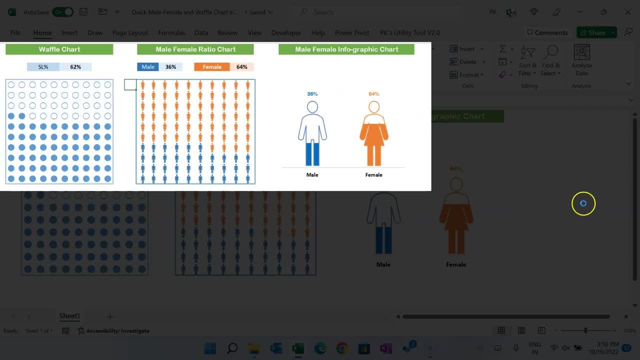 we are showing the male and female infographics, the field infographics, basically, And whatever the percentage, like 60% for the male. so 60% it is filled and this is 40% filled, All right, So I'll quickly tell you how you can create this using the quick trick in Microsoft Excel. 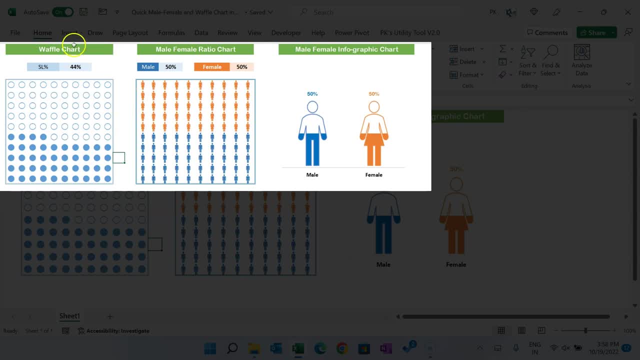 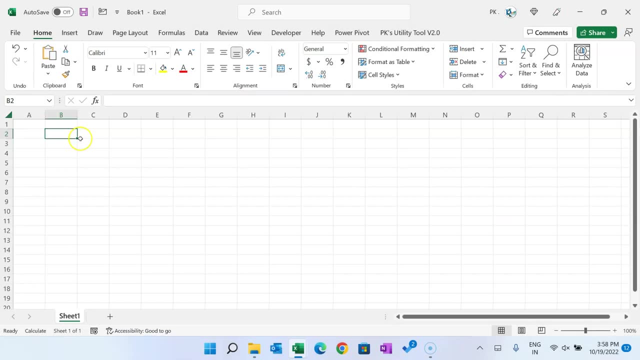 these three charts. So let's start without delay. First I will tell you how can you create this VFL chart. So let me add a new workbook: press control N. So let's say we are showing the service level value, and I'm putting here random value. 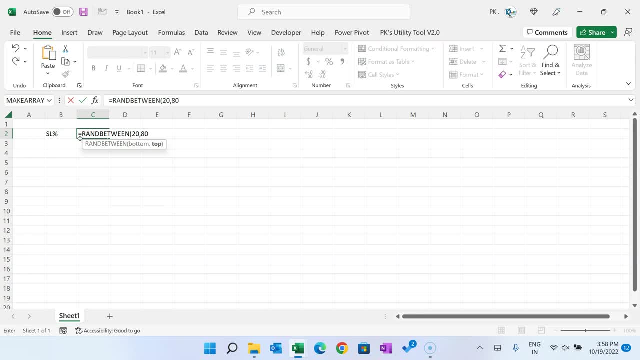 Let's say 20 to 80% of service level. So I'm putting here percentage sign Randomly. it will give some value. You can connect it with your original number. But here I'm taking the random numbers All right Now to create the VFL chart. what we can do, we can use. 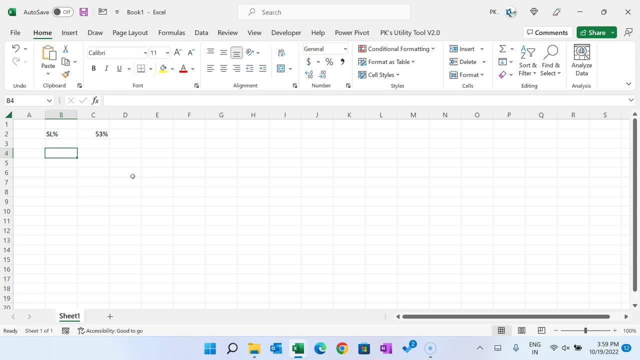 here sequence function, So let's use here sequence And number of rows. we will take 10 columns and just hit the enter So we can see the number from 1 to 200 here. Now we want to make it in the descending order. 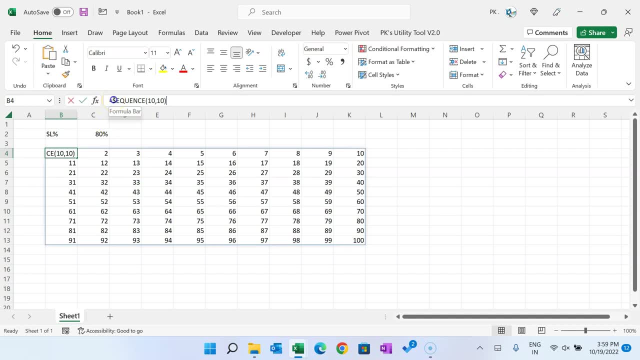 We can use the sort function before the sequence functions. Let's see: Use the sort functions, sort, and in the sort we will provide the array which can be the output of the sequence function. Then next is the sort index, which is optional. So you 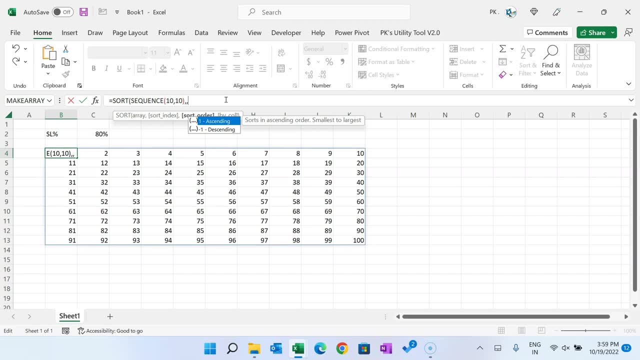 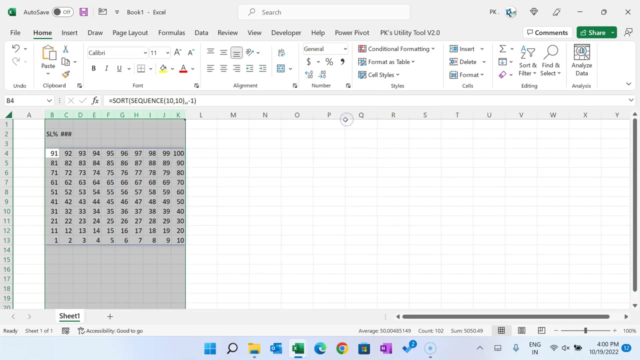 can ignore this. the next is short order. let's take it descending and just close the bracket. hit the enter. now we can see our number in the descending order. 1 is coming here and 100 is coming here. all right, now, we will arrange this in proper way. select all the columns. make the column bit slightly smaller, like. 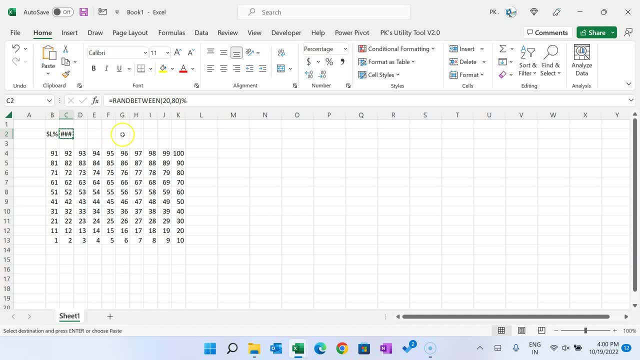 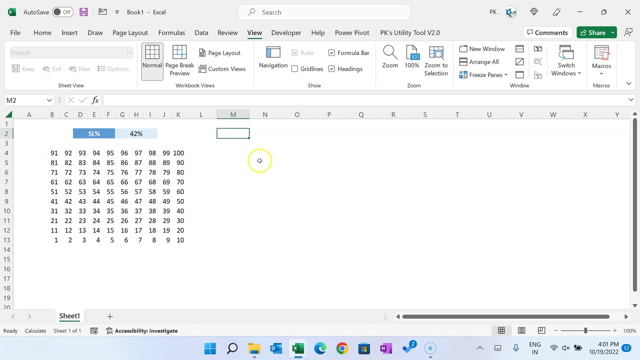 this and you can put your service level value somewhere here. make these three cells merge. put service level here and these three cells merge. go to the view and go to the show grid lines. let's uncheck this, so grid lines are not visible. now we have this number from 1 to 100 because we have 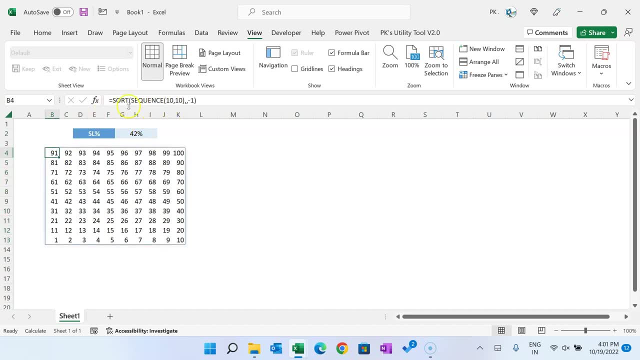 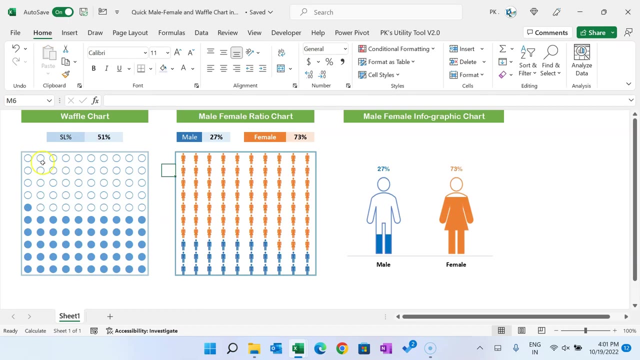 this number from 1 to 100 because we have our service level value in percentage, so we will show this value also in percentage. so let's divide it by 100. now it is in the percentage or decimal. now, here, in place of these numbers, we will show some icons, like here we have. 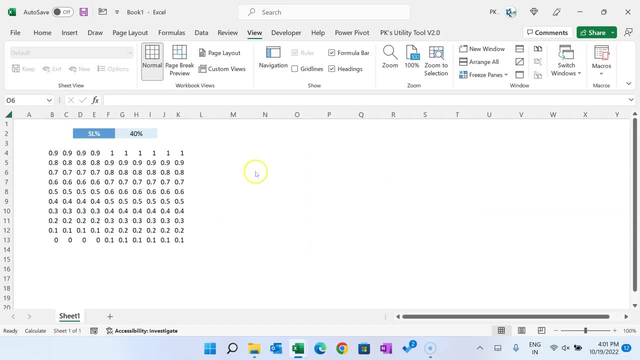 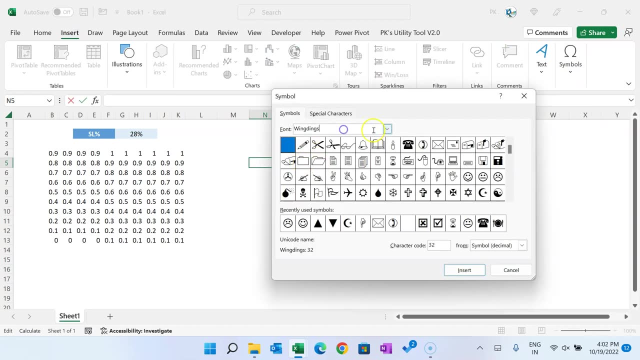 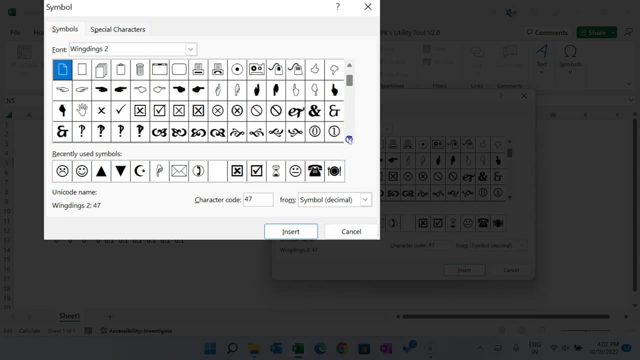 displayed these circle icon. all right, so what I will do here: I will go to the insert and then I will go to the symbols here and I will select here: bring brings to this one and here we can choose some icon. you can take these square also, or you can take these circles, or you can choose some other. 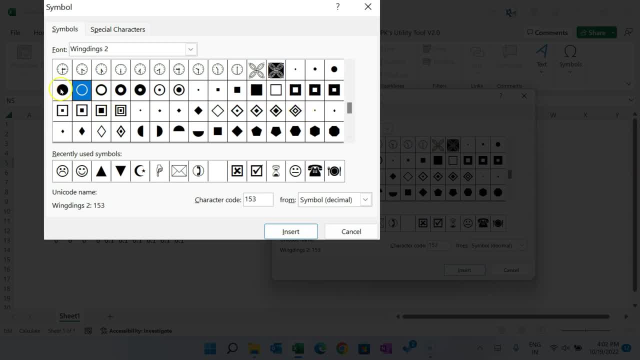 icons, whatever you want to choose. but here what I am doing, I am taking these circle icon. the first one- here you can see the character code is 152 and the second one is the 153. if you want to take the square, you can take 162 and the. 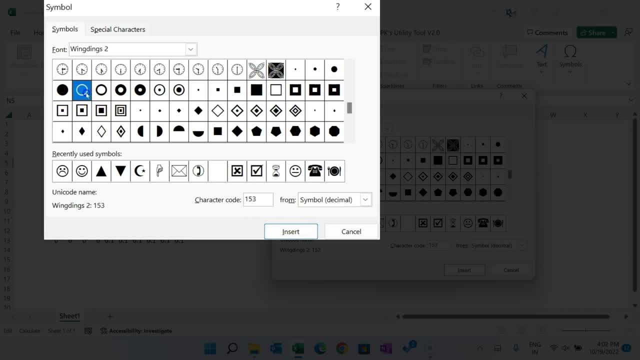 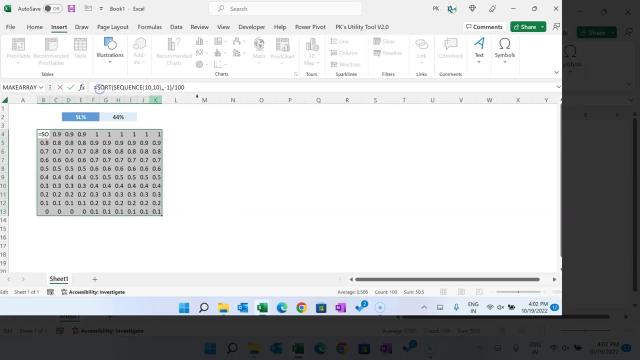 163, let's take here 152 and 153, all right, so I will put the formula here before the sort. let's put if condition: if output of this sequence function is less than this value, which is this service level value, as f4, then we will. 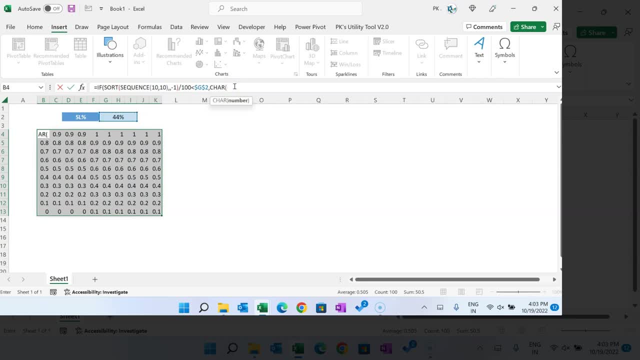 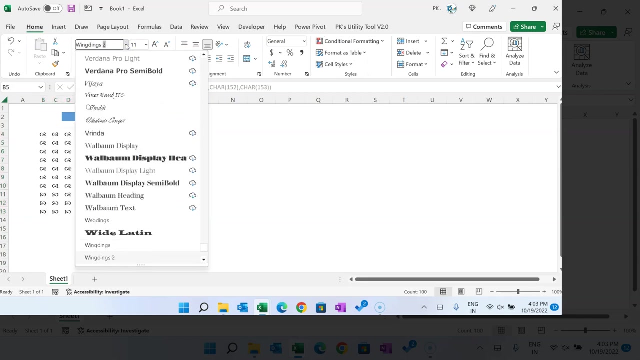 put here character and we will take here 152. let's close, else case we will take character 153. all right, now let's hit the enter and now I'll go to the home and I'll change the font here. I'll take the binding to. just type here: binding to. 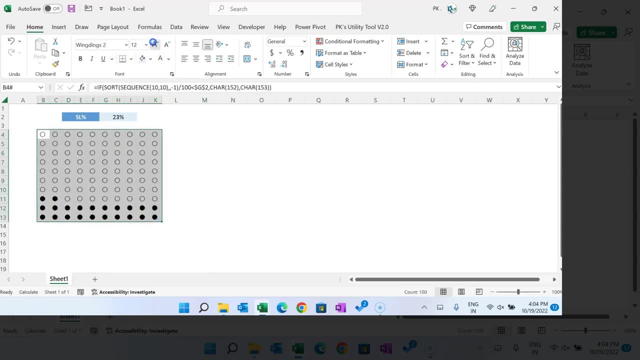 and just hit the end. now you can make it slightly bigger, the font size. let's take around 12. if you want to put some color, you can change the font color. let's say blue color. I have taken this one. you can put some thick water also you can take. 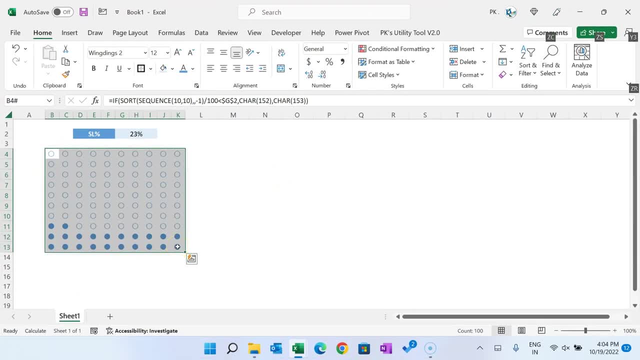 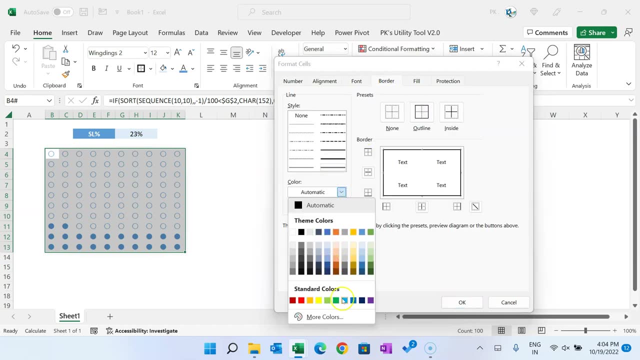 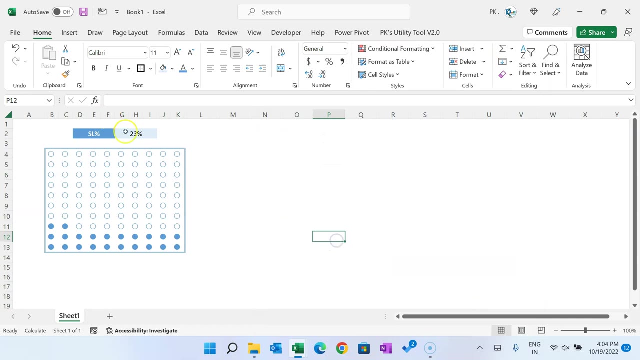 this one, or select this. press alt o- e to go to the format cells and then go to the borders. from here you can choose this border. let's take the color- also this color. then choose this water. click on outline. okay, this is ready. now, if I will, 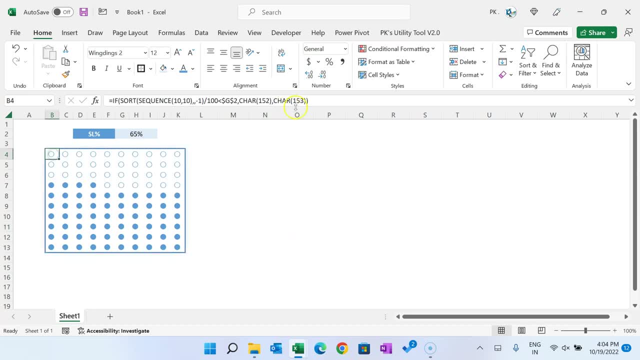 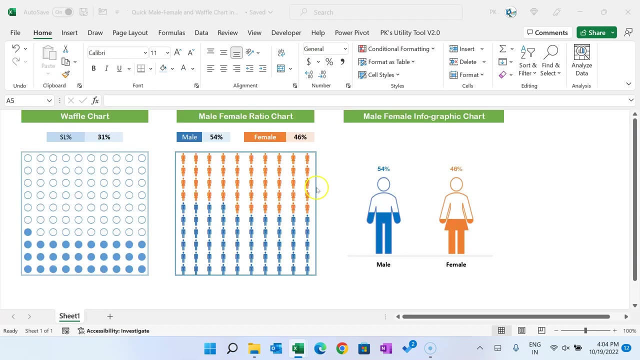 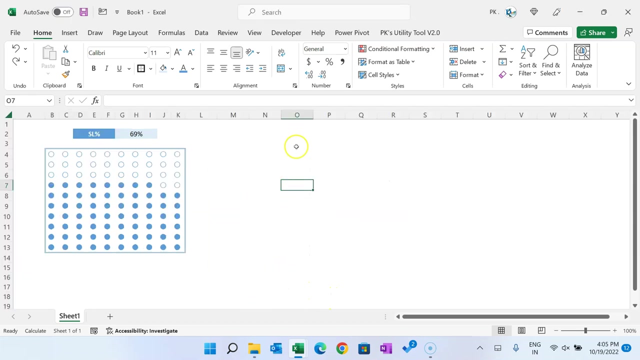 refresh, then you can see it is getting changed. similarly, you can change the characters by 162 and 163 also, like this, so it will show the squares in place of circles. all right, now I'll show you how can you create this male- female chart. also, we are using the same thing here. we have put the friend between function, so 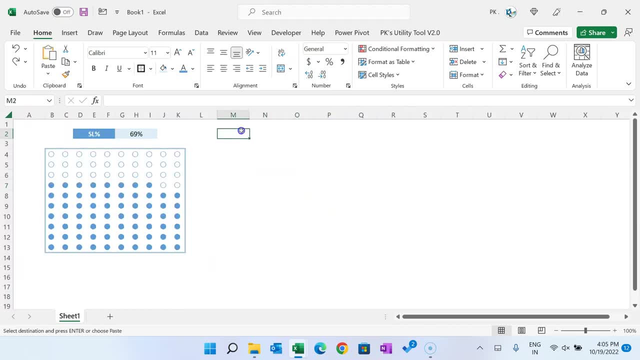 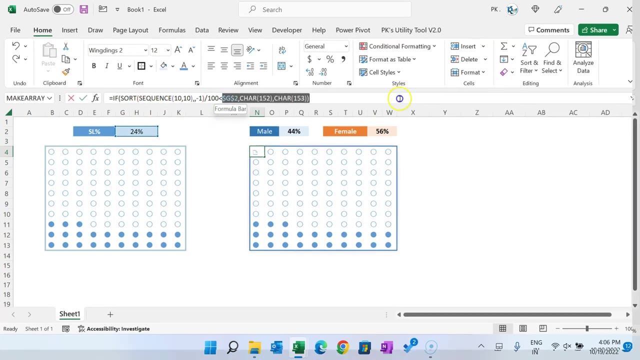 let's copy this and just paste this here, right, and we will make smaller the size and we can copy the same formula which we have done here. let's paste this here. we will make the changes in the formula. so let's delete the formula from here. we'll keep this formula only, and let's put here: 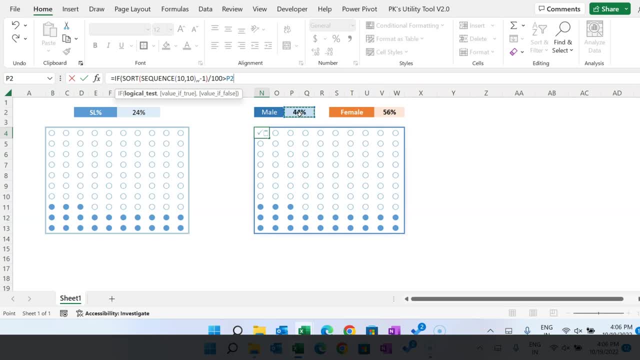 if this value is greater than this value, which is male percentage, press f4 to freeze this. then we will take character 129 and then we will take the character 128 and these character 129 and 128 for male and female and just close the bracket and hit the enter. you can select this and. 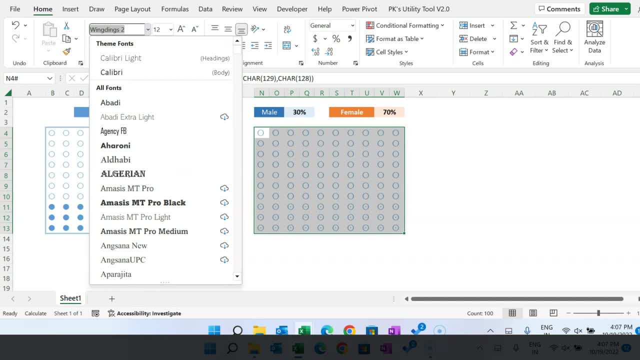 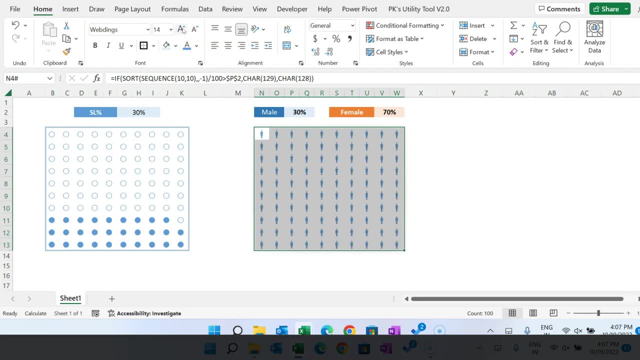 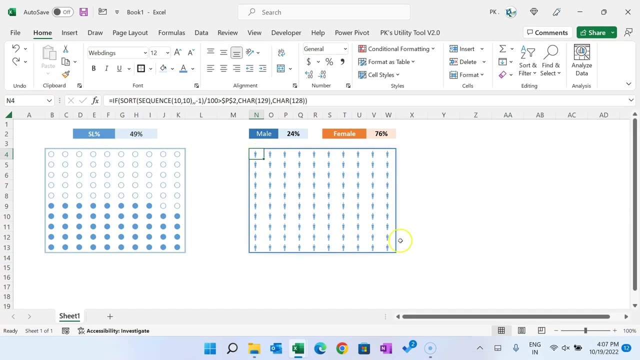 change the font as labedings, so let's select here labedings. you can see the male and female icon there. it will make slightly bigger. we can put here conditional commenting because we want to highlight the males and females separately. so let's select this range. go to the home and conditional formatting. let's put a. 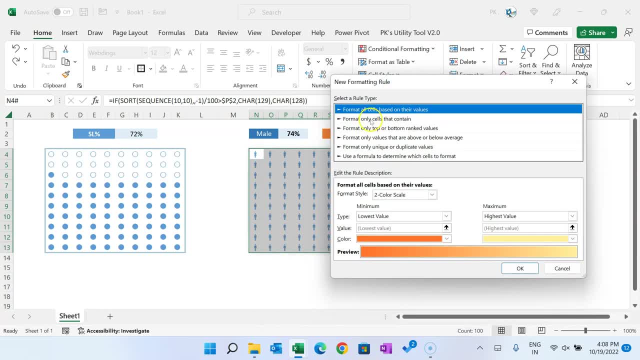 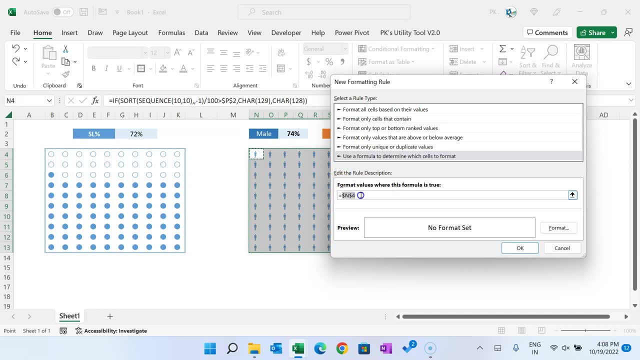 new rule and we will put here a rule. go to the use a formula to determine which cell to format and just select this cell. we will not take the dollar sign, so just press f4 price. if this value is equal to character 129, then we will format this. 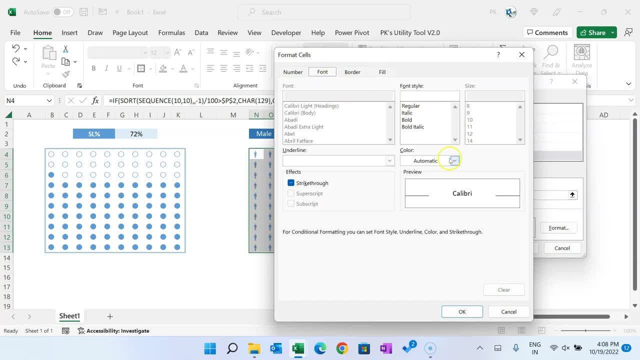 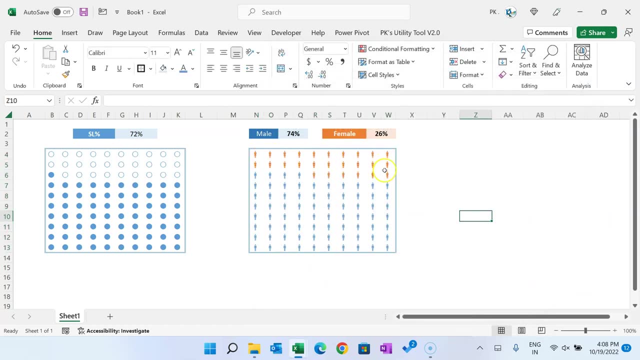 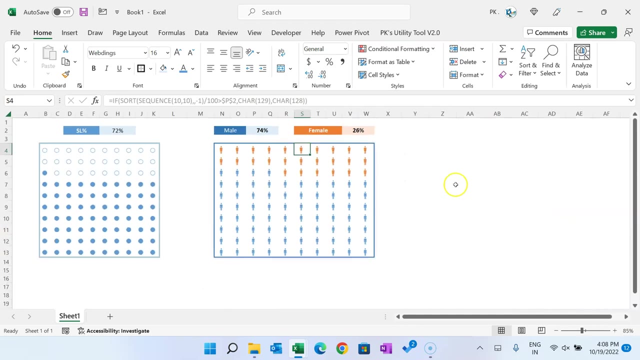 let's say in this color. so change the font. only now, just change the font. only now, just change the font. only now, just this one, okay, okay. so here you can see, the females are highlighted in the different colors and males are in blue color. alright, friends, so that is how you can create this chart. now I'll show you. 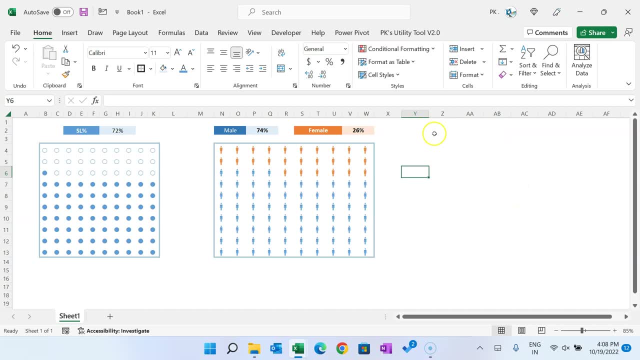 quickly, how can you create the male and female infographics chart? let's put here male, and this can be for female. let's put here max value. okay, now, for male, we will take this value and for female, we can take this value and max value, we will put here one which. 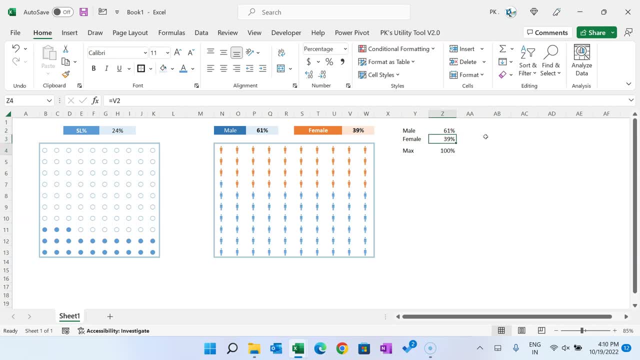 is 100%, okay, or you can put the max value for male and female both in front of this one. so let's put here 100% and here also 100%. so this is actual value and this is maximum value. alright, let's select this and go to the home and go to. 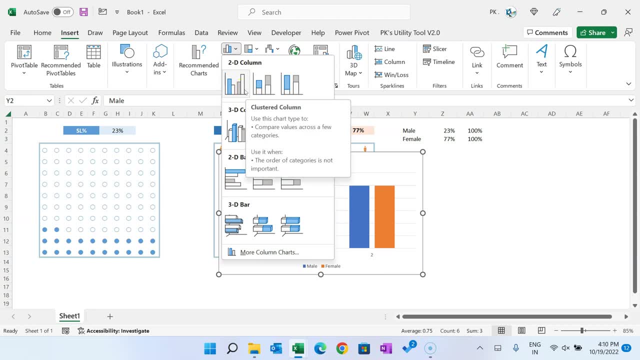 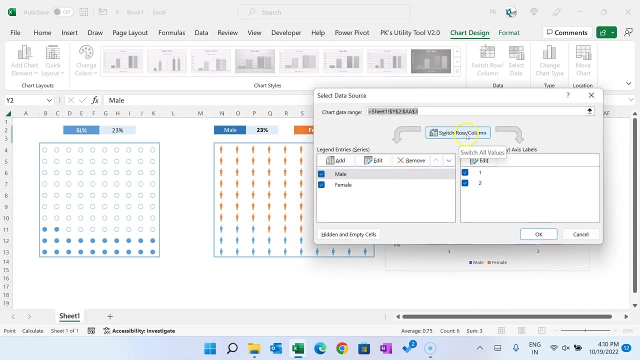 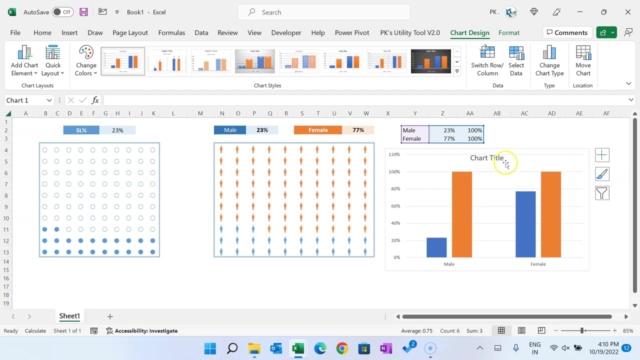 the insert chart and we will take this chart, which is cluster column chart. now right click on the chart and go to the select data and here just click on switch row column. click on ok. now our chart will look like this: delete the legend as well as the chart title, and you can remove the grid lines from here. 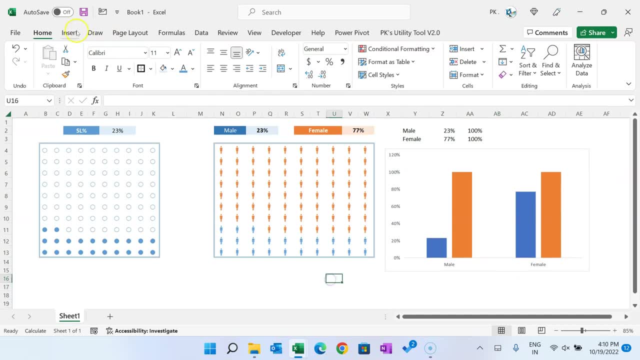 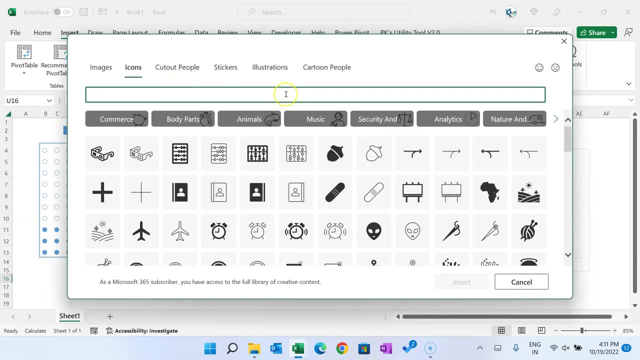 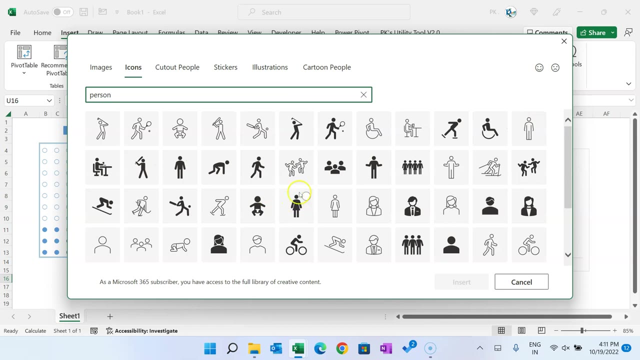 alright, now I'll go to the insert and I'll go to the icons. let's insert icon. and here we will insert the icon for male and female. you can search here for the person and we can choose male and female. let's take this one for male. let's take. 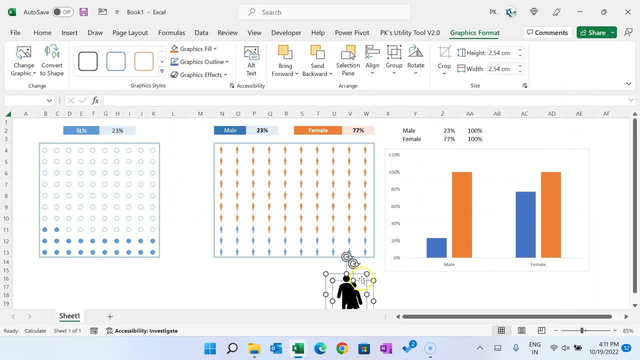 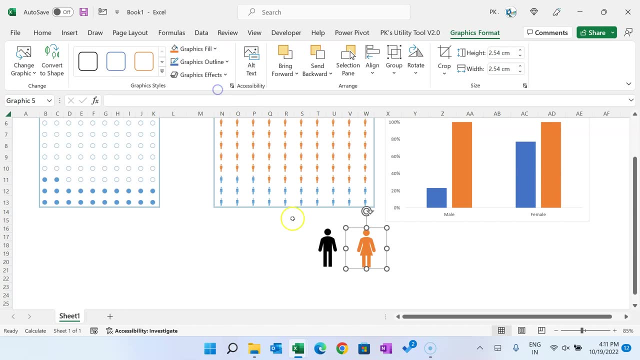 this one for female. so these two icons insert. we have both icons here. we will fill some different color. for female, let's fill this color, and for male let's fill this color. select both the icon, make the copy of those and just keep this here now. in the second female icon we will fill no. 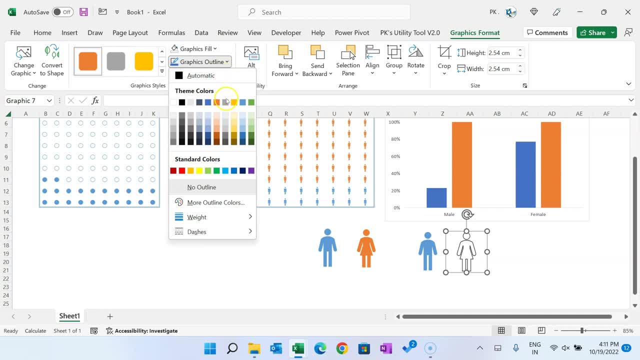 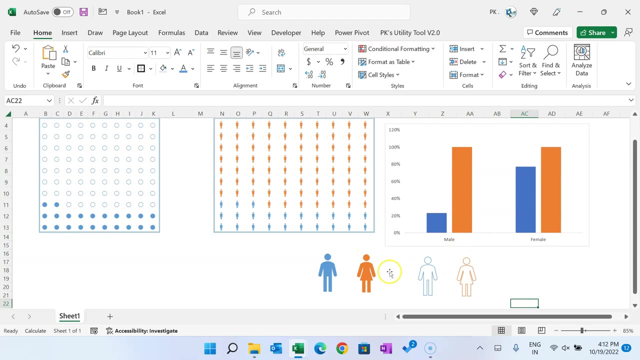 fill and the graphic outline. we will choose this one. and here in the male, we will choose no fill and graphics outline. we will choose this one. alright, so basically we have one filled and one not filled icon for male and for female. so let's copy for male this filled icon. copy and select this. 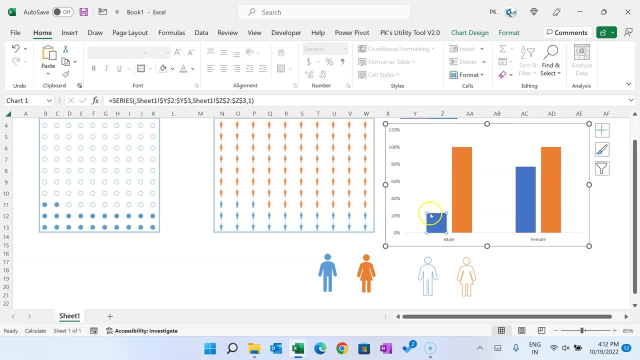 one for male. click again so that only this will be selected, not this will more selected, and paste that icon here. now right click, go to the format data point, go to the fill and line here, go to the picture or texture fill which is already filled, and now select here stack and scale width. make sure units slash. 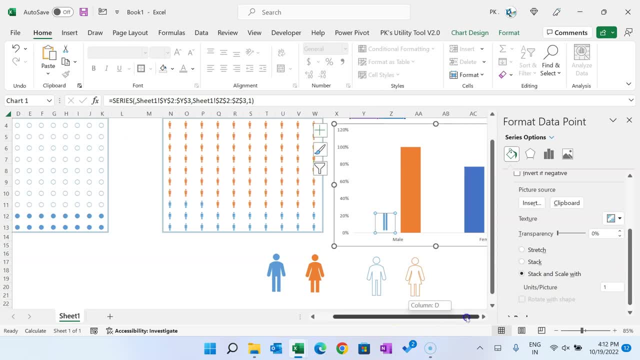 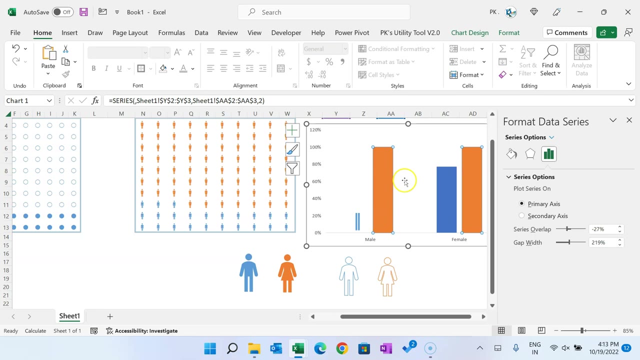 picture should be 1, which is already there all right now. copy this unfilled icon for male and paste this here. select only this one. so to select this you have to first you will click here, both the orange selected. just click again on this, then only this will be selected. paste. 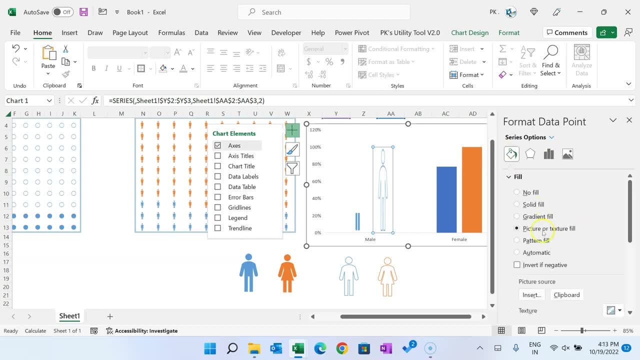 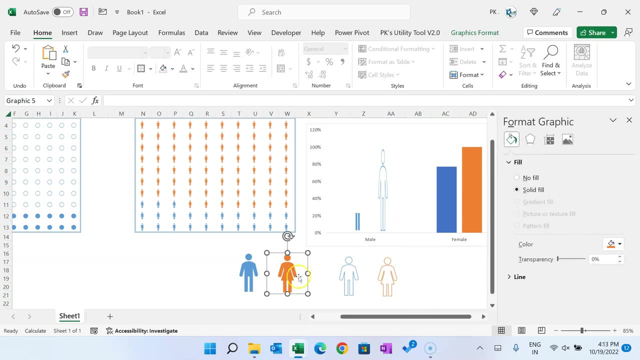 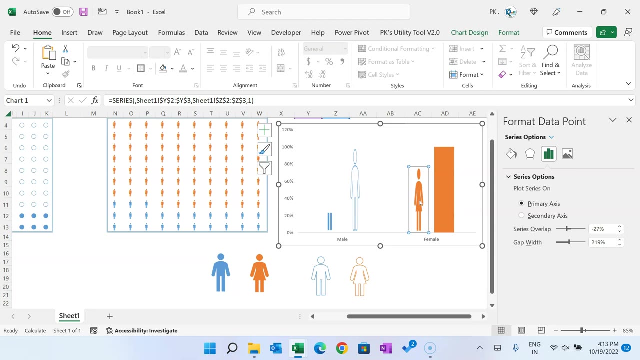 this here. go to the fill picture and again stack and scale. all right, similarly we will select for female. also copy this. come to the female below this one click, double click here and paste and go to the picture and line picture and select here, stack and scale with. now copy this icon and just paste this here. 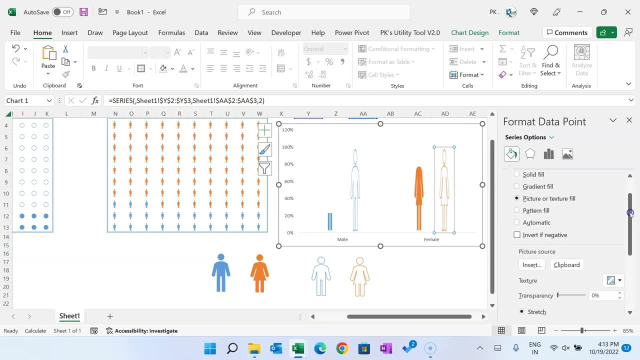 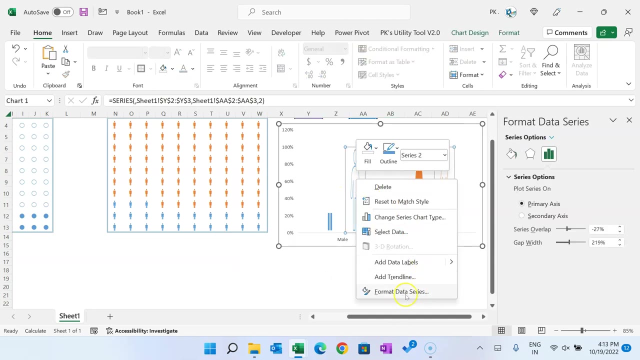 go to the fill and line and come to the pictures or texture, fill, stack and scale. with that's it. now we can remove these icons left and press delete, right click and go to the format data series. here we cap it. let's take zero and the series overlap. let's.